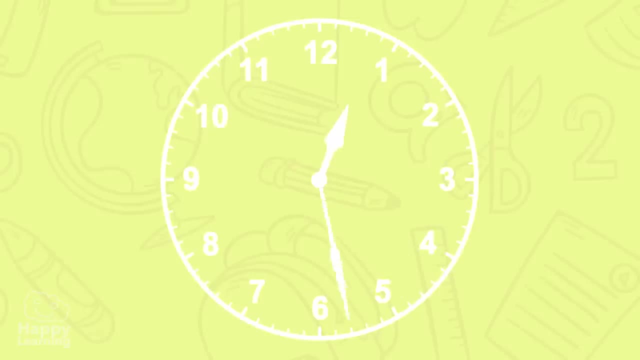 If you look around, we are surrounded by angles Like the ones this clock handles Or an ice cream cone makes. The unit of measure of the angles is the degree, And the most important angle of all is this one. It's called a right angle and it measures 90 degrees. 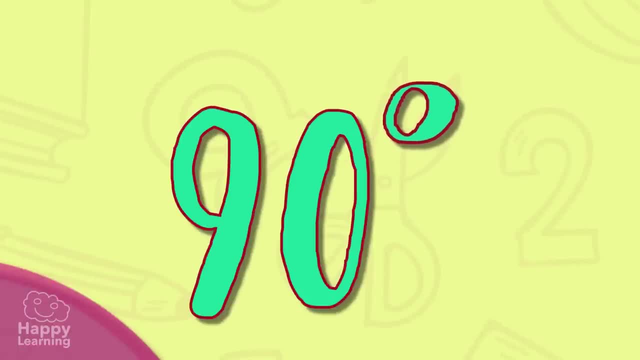 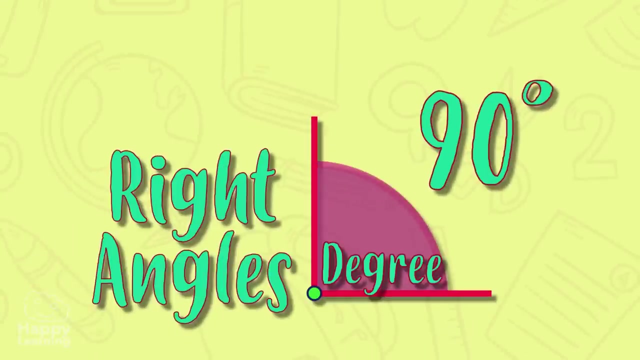 The tiny zero you can see in the right upper part of the number 90 is a symbol that represents all angles. We say that a right angle is the most important one Because it is the one that is used to compare all of the other angles. 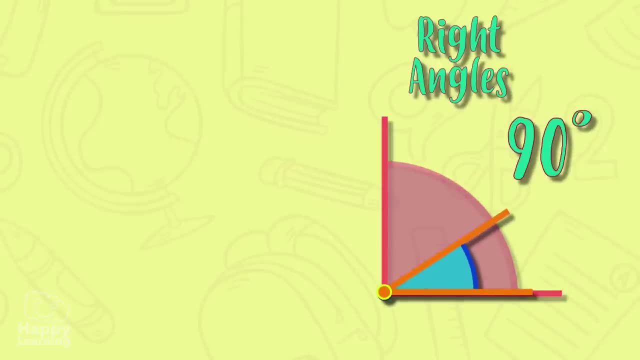 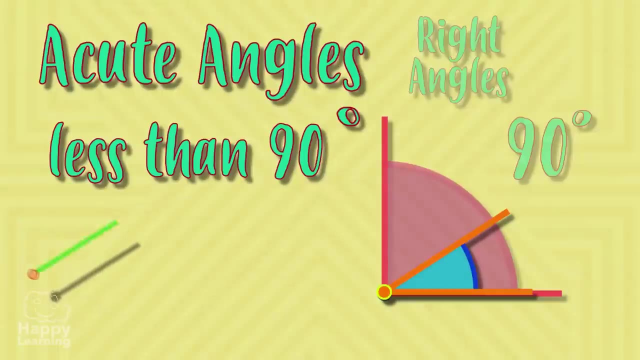 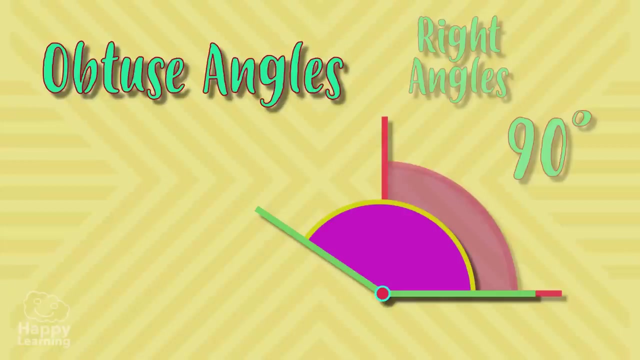 The angles that are smaller than a right angle are called acute angles, And they measure less than 90 degrees. like all of these. And the angles that are bigger than a right angle are called obtuse angles And measure more than 90 degrees. like all of these. 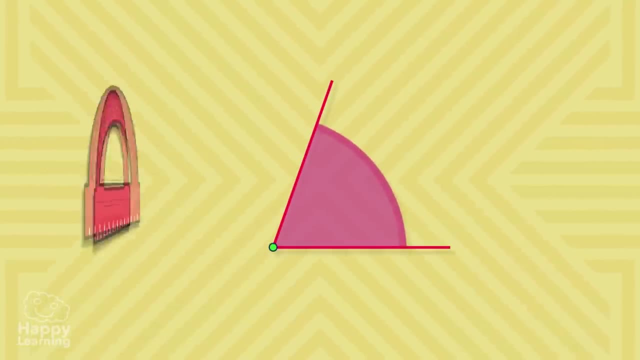 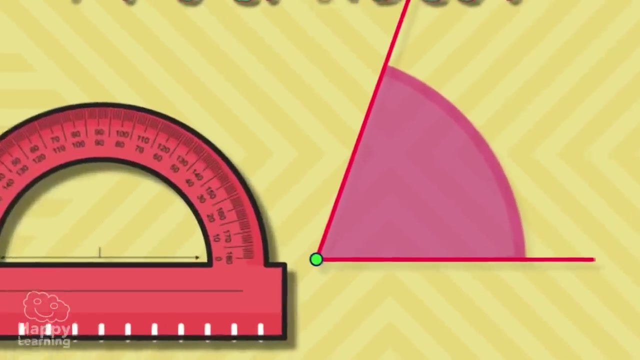 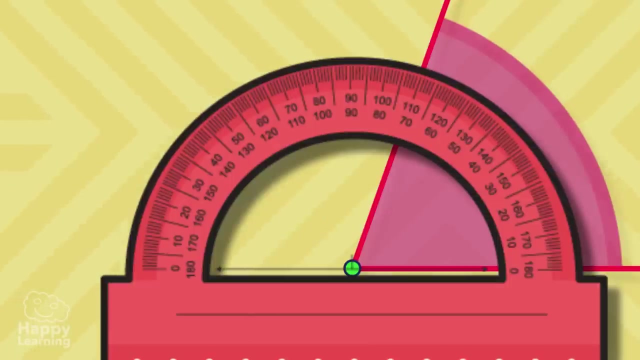 To know the degrees that an angle measures, we need to use this instrument, Which is called a protractor. So we need to place the straight part of the protractor over one of the sides of the angle, Making the vertex and the central point of the protractor meet. 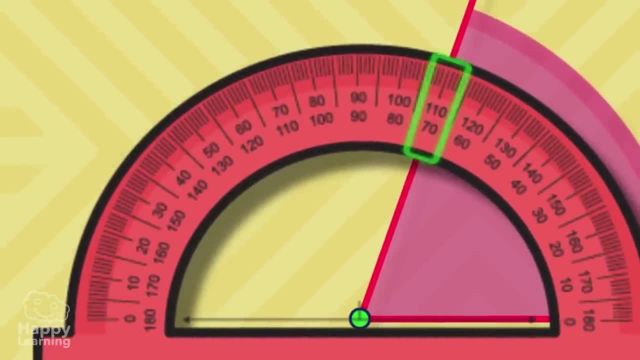 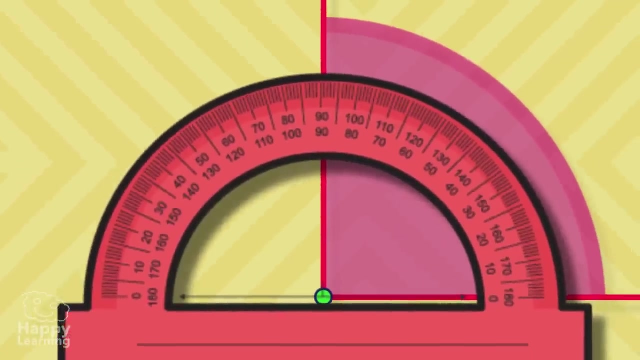 After this, we need to look at the protractor line on the other side of the angle And look at what number it says. These are the degrees that an angle measures. Easy peasy, huh, Let's practice. We said that a right angle is 90 degrees. 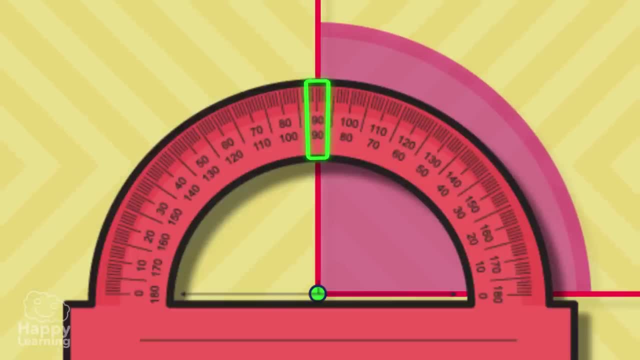 Let's see. We'll get the protractor and, Indeed, A right angle is 90 degrees. We haven't fooled you, huh. Now Let's measure this angle. Let's see how much it measures. 45 degrees: It's an acute angle because it is smaller than a right angle.